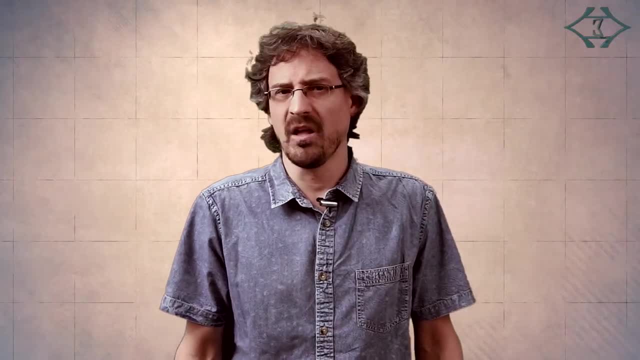 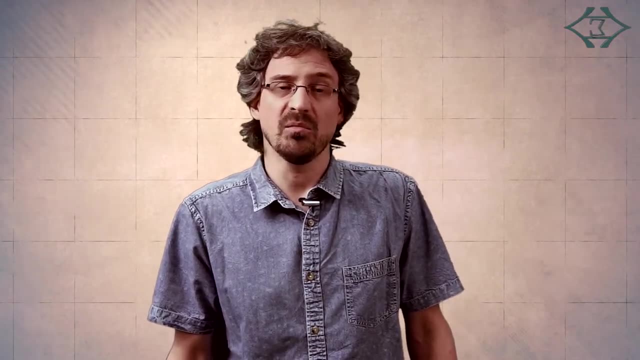 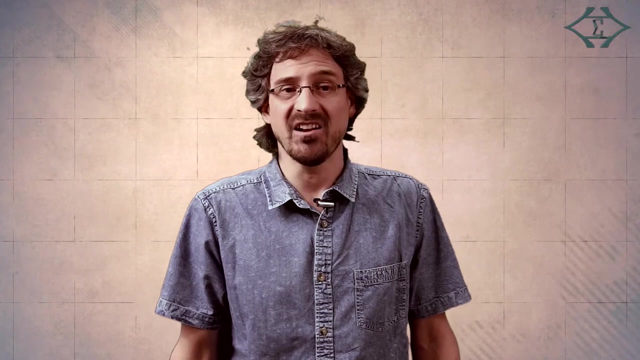 which a conclusion can be derived from. Thus, we often use the words premise and proposition interchangeably. Another word which is sometimes used instead of premise is statement. Consequently, during the most part of this and subsequent videos, we shall be using such words as premise, proposition. 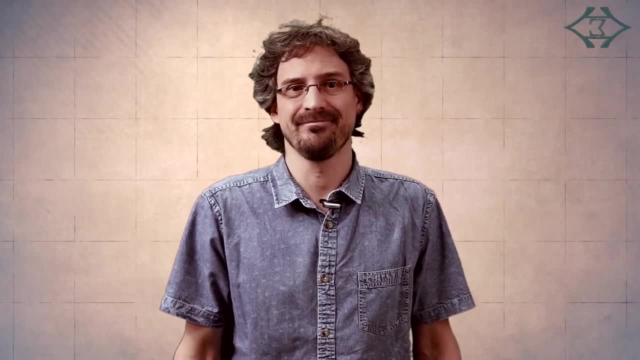 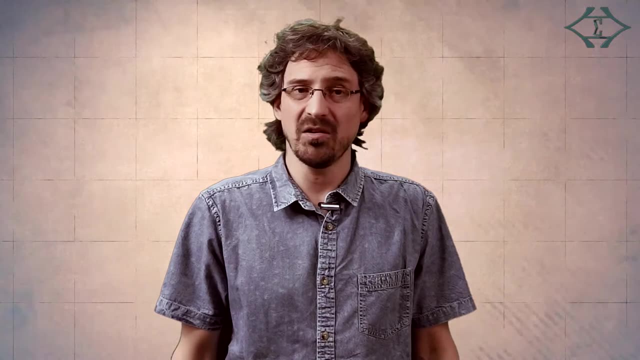 and statement interchangeably. Now, in logic, a premise, proposition or otherwise, a statement is a sentence which has an unambiguous interpretation of being true or false. So it's worth mentioning that the regular Janis and Janis 한� trespassieren nicht. 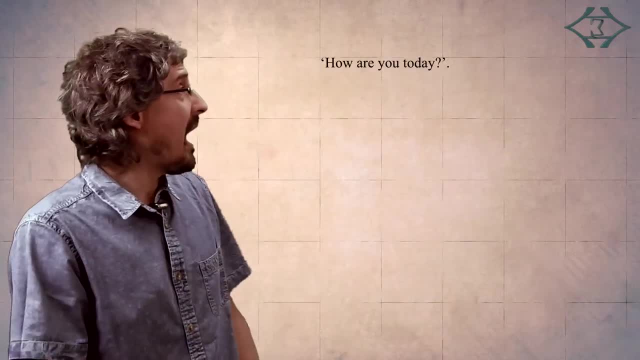 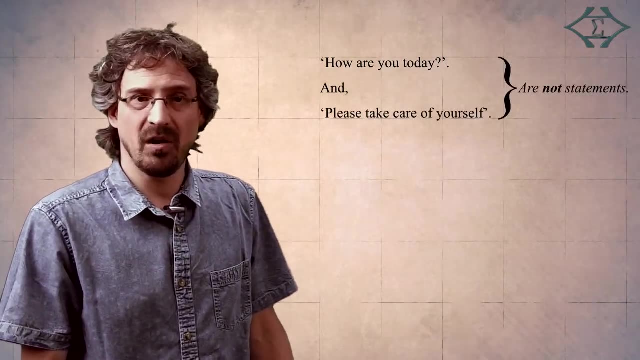 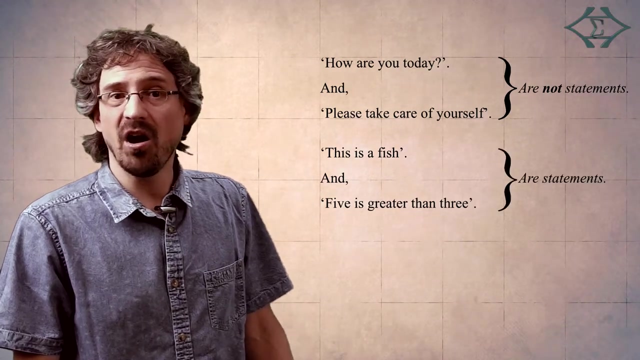 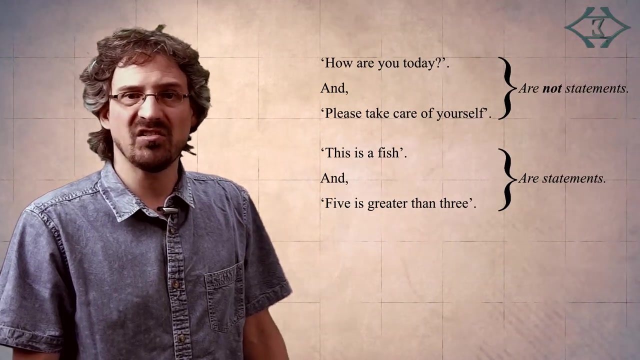 or false. Thus, sentences like how are you today and please take care of yourself are not statements. Where sentences like this is a fish and 5 is greater than 3 are statements, since, regardless of one's knowledge of fish or that of numbers, there exists a notion. 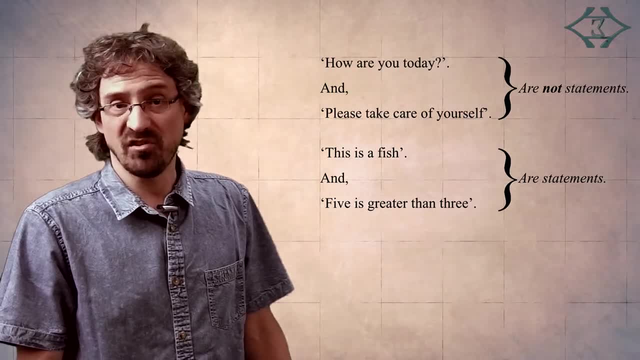 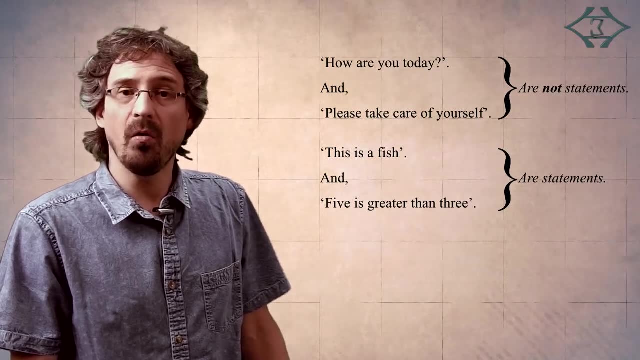 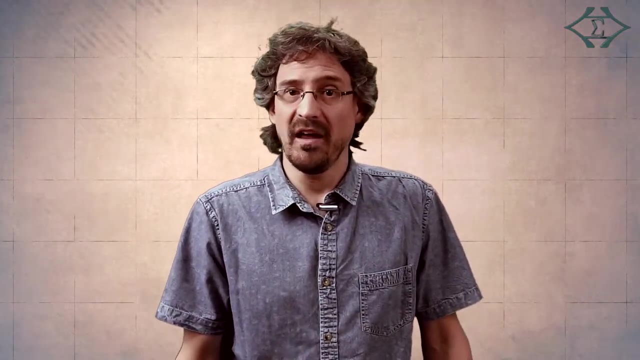 of being true or false, And so propositions are those sentences that we can assign a truth value, which is either the truth or the false. A logical deduction, on the other hand, is the formal process where a conclusion is obtained from known statements in force. We often describe: 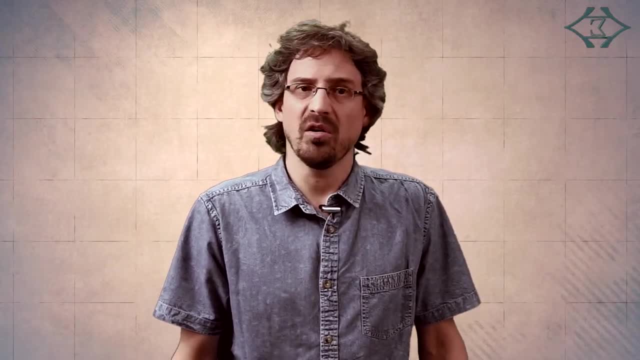 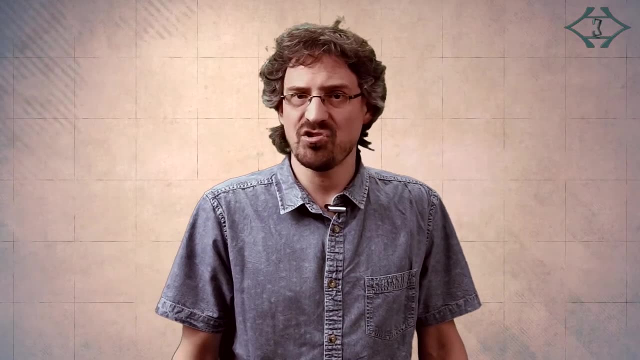 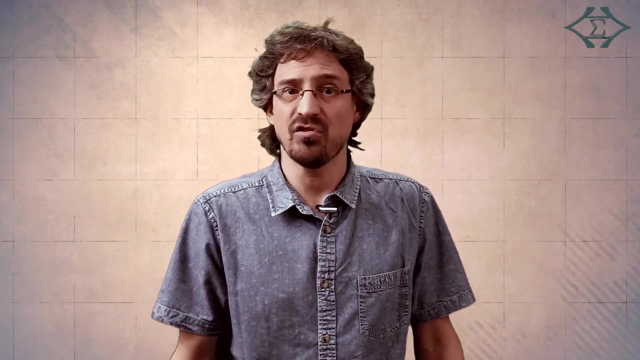 logical deduction as truth preserving. This is because deductive logic is characterised by what is known as Logical Validity. In the aforementioned video, where we introduced the basic concept of deduction, we defined logical validity as where the truth of the conclusion is guaranteed on the proviso that 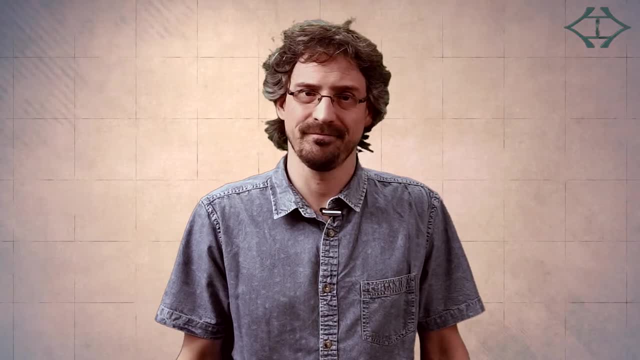 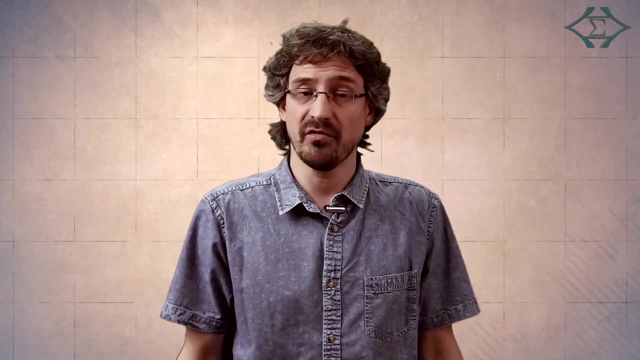 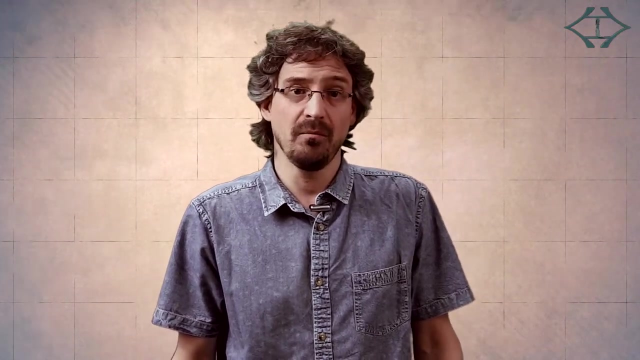 the premises in force are true In many situations. if new results are sought from a particular branch of mathematics, then a process of analysis becomes a plausible discovery. A process of analysis will often include some special cases of interest. first, Mathematicians are frequently referred. 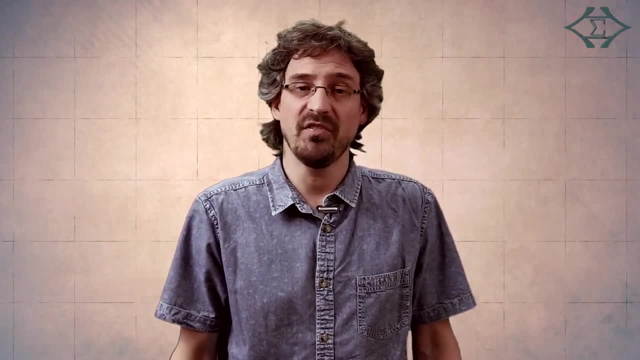 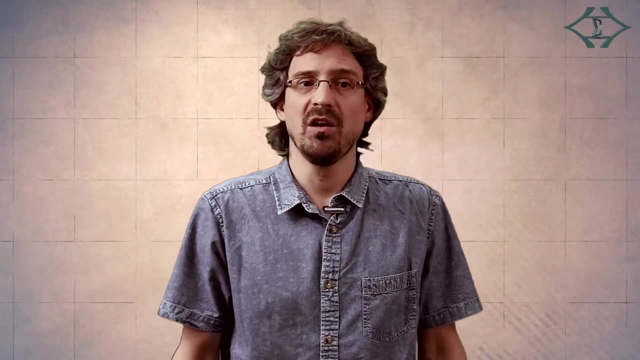 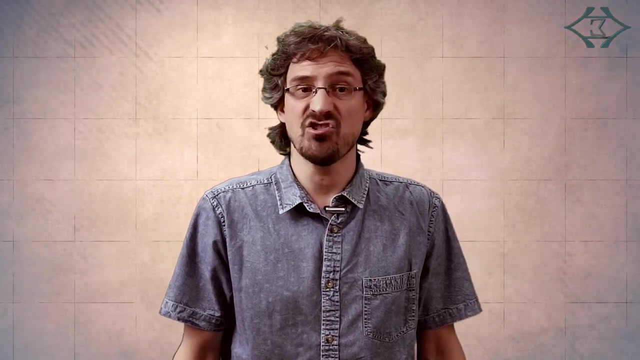 to as pattern hunters. This is because of the investigative nature of the analysis, which can reveal mathematical structures or patterns where a mathematician may be able to establish a possible rule. Such a proposition is called a conjecture. It is now the job of the mathematician. 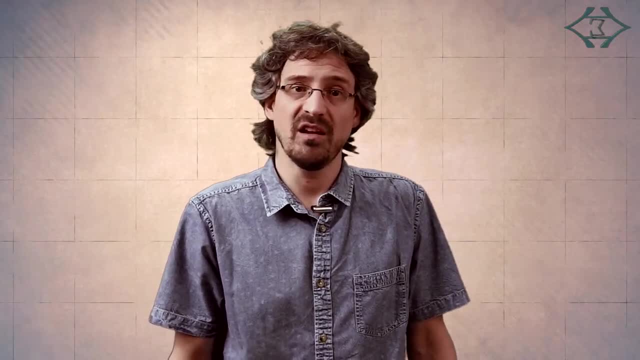 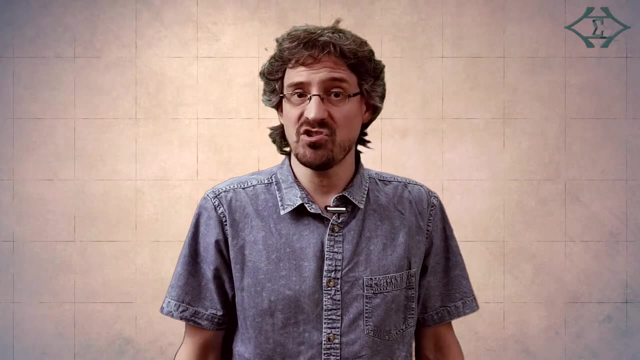 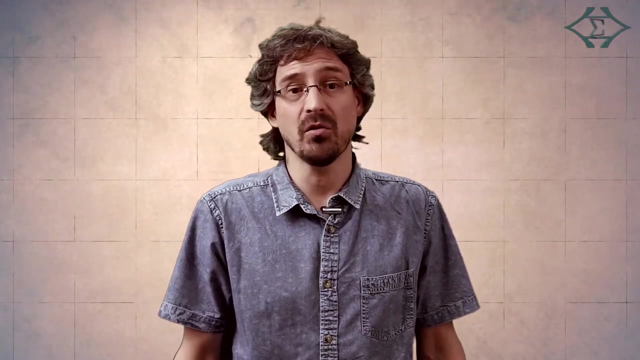 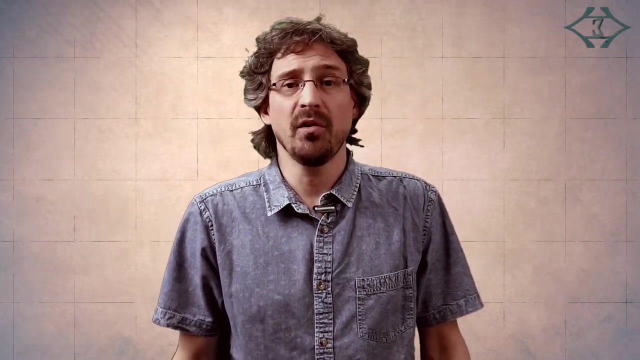 to ascertain a logical process introducing its truth, thereby establishing a mathematical proof of the statement. With the successful completion of a mathematical proof, we can then elevate the conjecture to the status of a mathematical theorem. As a simple example of a conjecture in mathematics, suppose the following pattern of adding two: 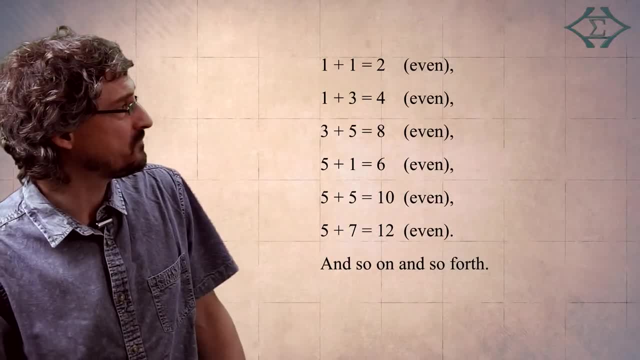 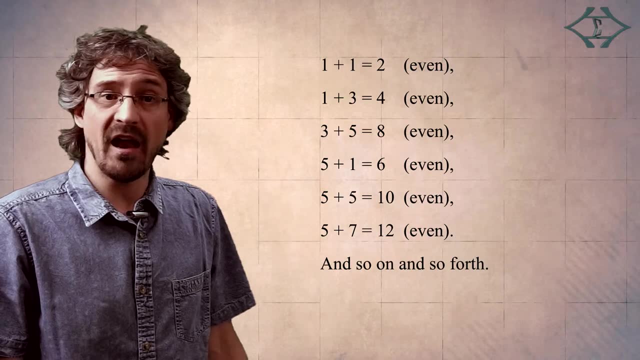 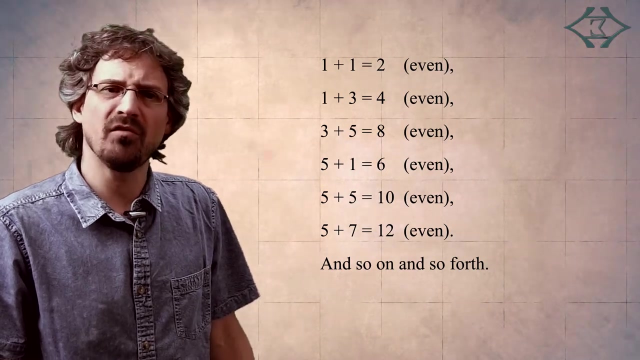 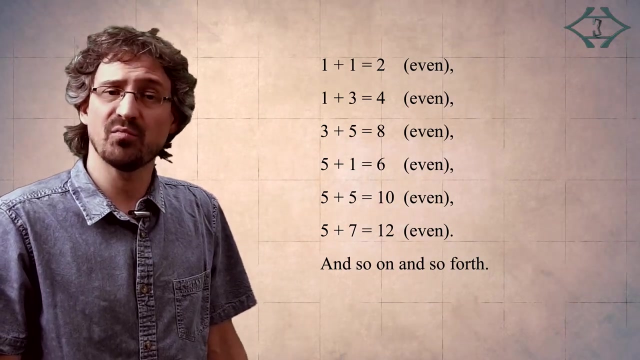 odd numbers together is observed. From this, it could be conjectured that the sum of any two odd integers is even. But how do we know that this is true? After all, we have not tried adding together all possible pairs of odd integers. To prove this, we require a way of expressing mathematically. 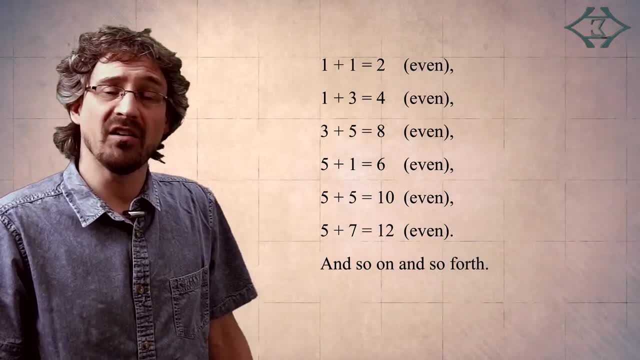 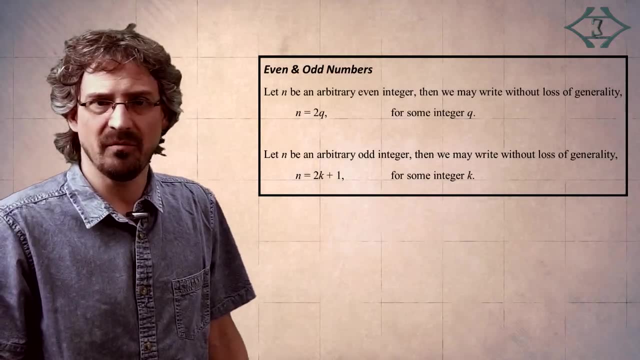 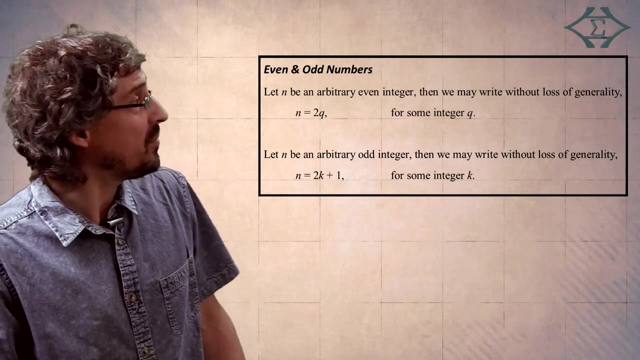 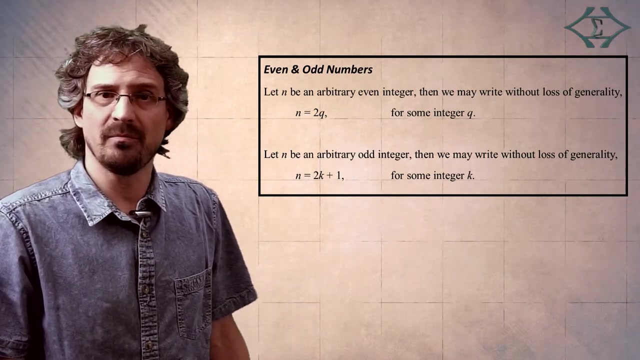 arbitrary even and odd numbers. And indeed there is a way to do this. Let n be an arbitrary even integer, then we may write without loss of generality: n is equal to 2 times q, where q is some integer. and let n be an arbitrary odd integer then. 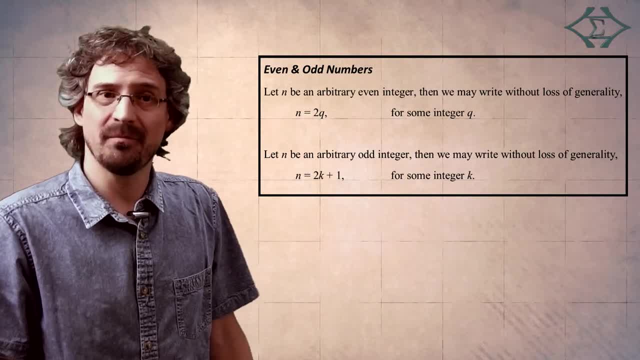 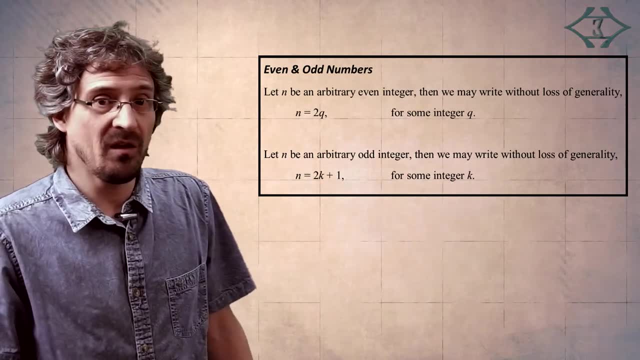 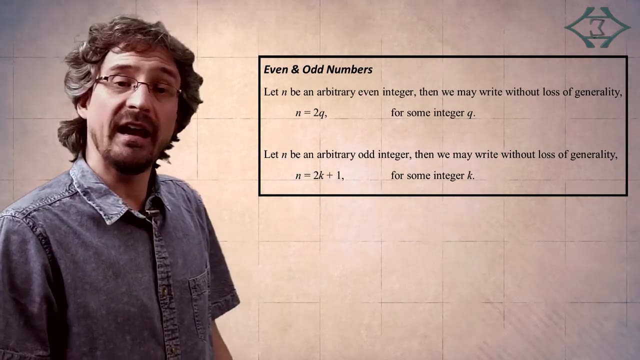 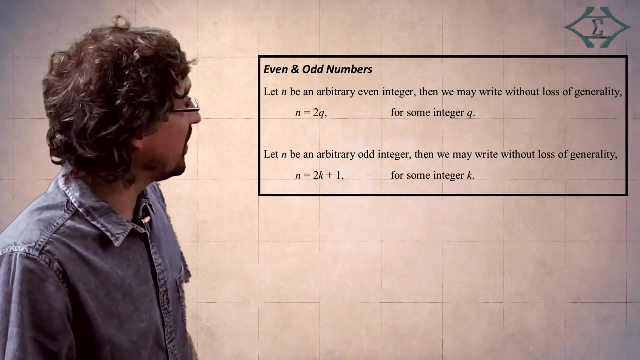 we may write again without loss of generality. n is equal to 2 times k plus 1.. For some integer k. In our introduction to number theory we should provide an explanation as to why this general form of even and odd numbers is justified. But the simple answer is: on dividing by 2,. 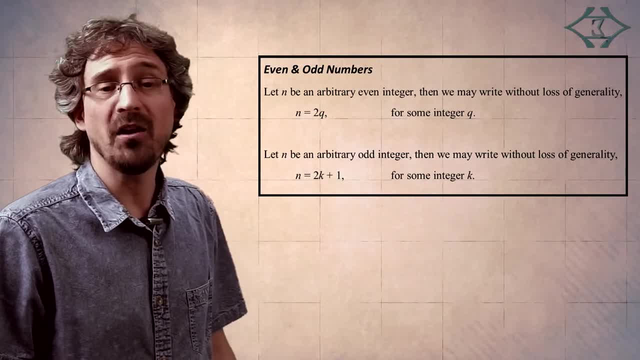 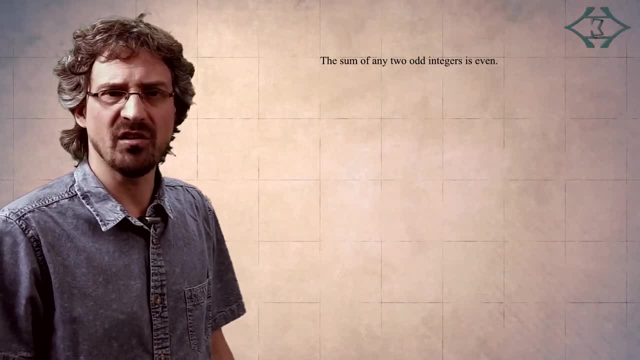 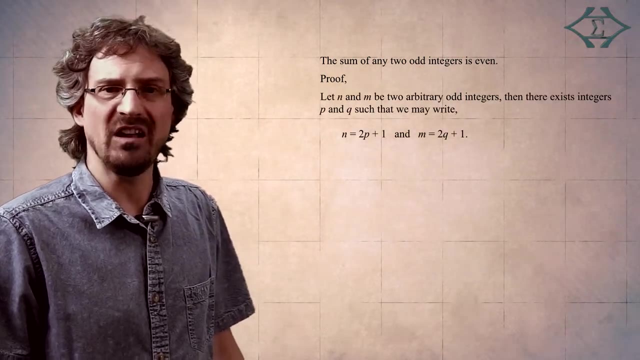 even and odd integers have a remainder of 0 and 1 respectively. We now prove the conjecture that the sum of any two odd integers is equal to 1.. Here's the proof. Let n and m be two arbitrary odd integers. then there exists integers p and q, such that 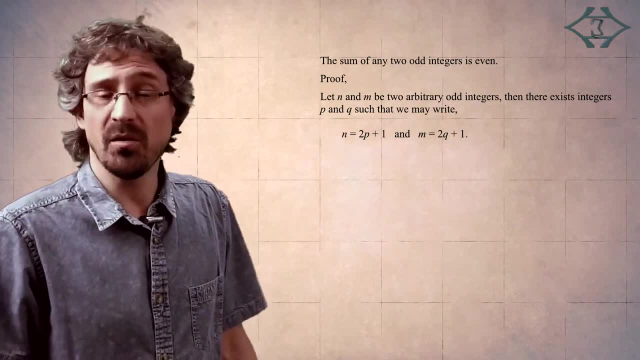 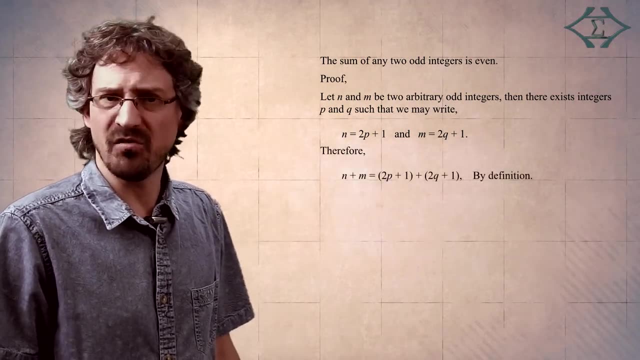 we may write: n is equal to 2 times p plus 1, and m is equal to 2 times q plus 1.. Therefore, n plus m is equal to the sum of 2 times p plus 1 and 2 times q plus 1. by definition. 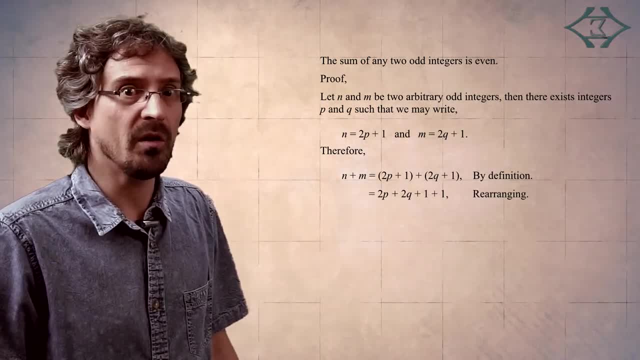 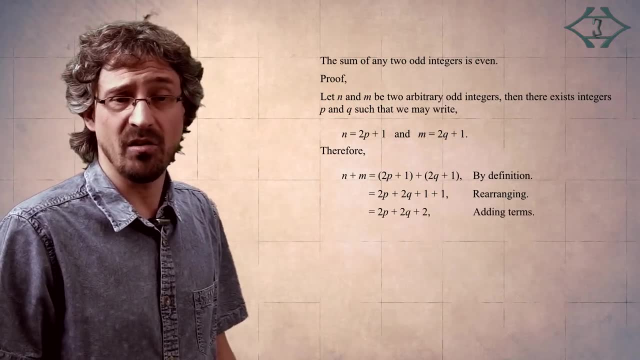 We can write this as: 2 times p plus 2 times q plus 1 plus 1.. Let's simplify that a little by adding the ones together. Quite superficial simplification, however, but that factorises by 2, so we obtain 2 all. 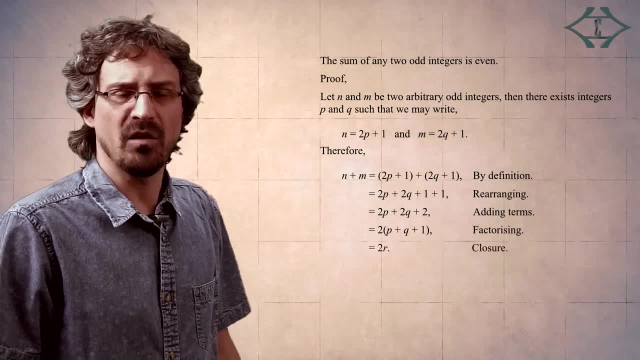 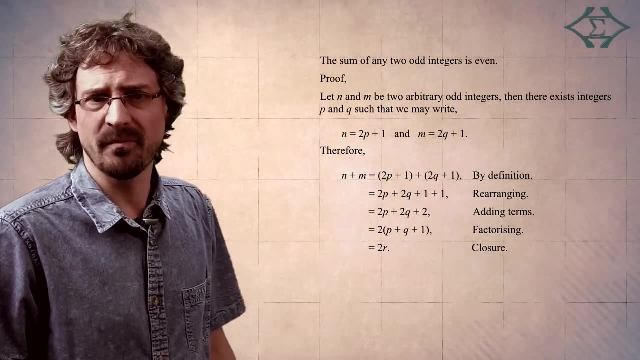 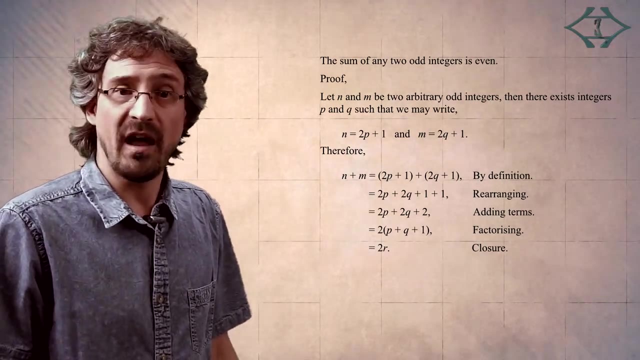 multiplied by p plus q plus 1.. We can write this, as a somewhat simplification, as 2 times r, where r is an integer. The final step in the equation: It's using the fact that the sum of any two integers is also an integer. 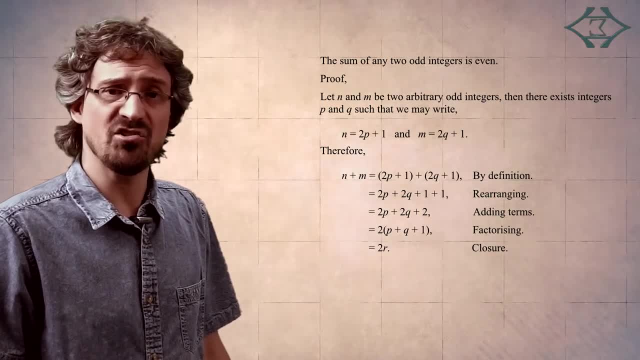 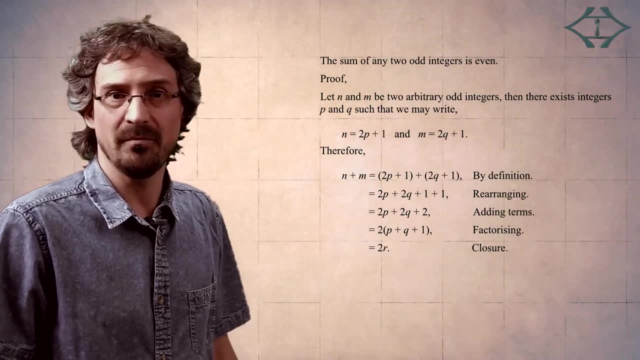 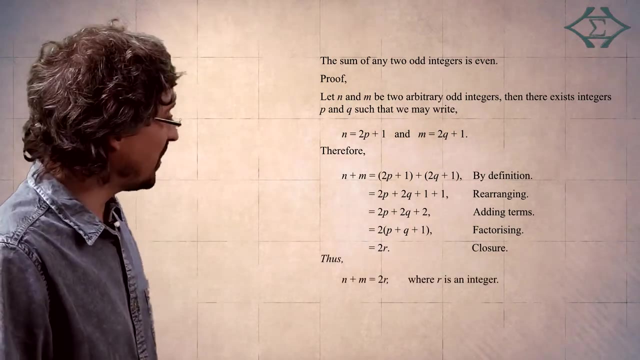 This is known as closure, That is, the set of integers is closed under the binary operation of addition, together with the property of associativity. Thus the result follows. Thus, n plus m is equal to 2 times r, where r is an integer. 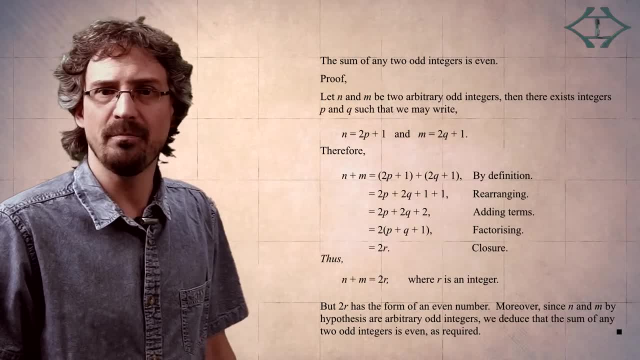 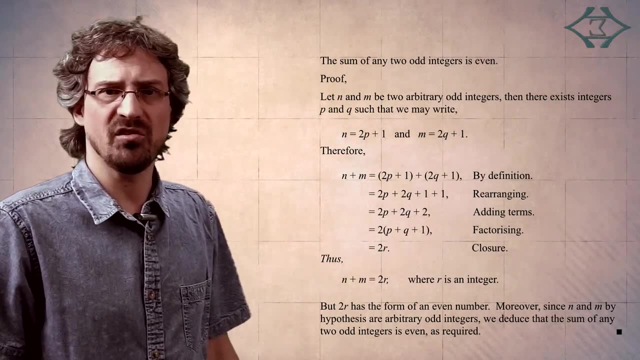 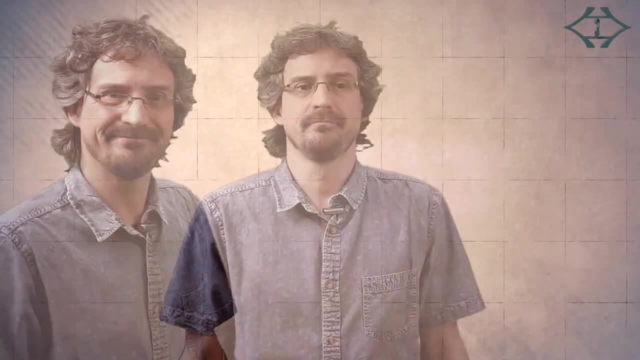 But 2 times r. The sum of n plus m has the form of an even number. moreover, since n and m, by hypothesis, are arbitrary odd integers, we deduce that the sum of any two odd integers is even, as required. Thus we have now proven the conjecture to be a mathematical theorem. 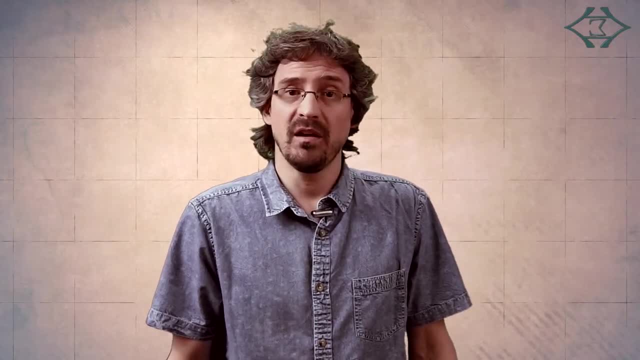 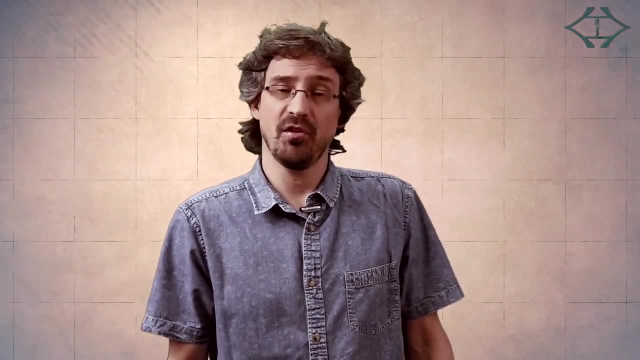 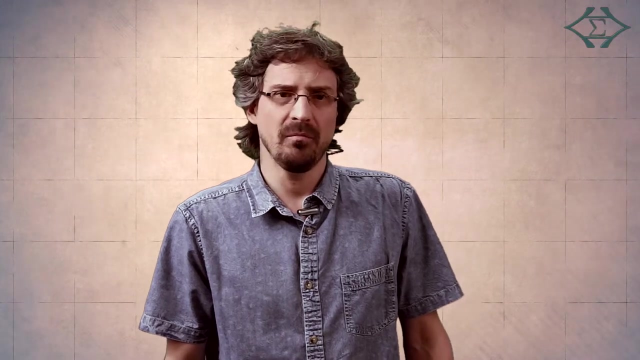 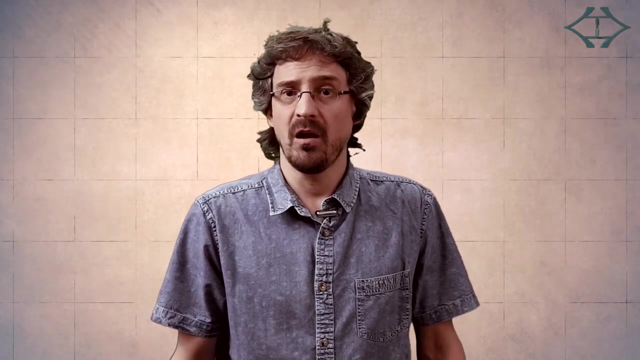 However, strictly speaking, the term theorem is usually reserved for a key result, one which is of significant importance. Other terms of a derived result in mathematics are lemma and corollary A. lemma is generally considered to be a minor result and are often used to derive theorems.